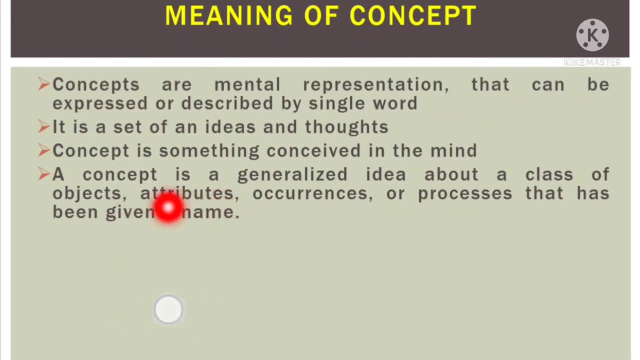 Attribute means the specialities or qualities of those objects. On the basis of those qualities, a group is formed. Occurrences means what has happened, what is happening. On the basis of that, a group is formed. And your process means what is the process. 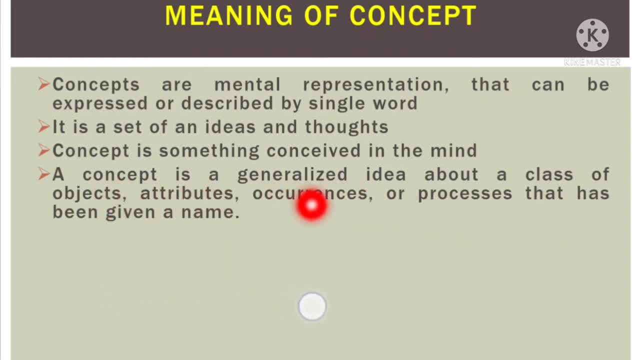 So if we talk about a concept, then concept is basically a journalised idea In which we consider some things: What is its class of objects, Means, what are its properties, What are its common properties, Or what are its attributes, What are its specialities? 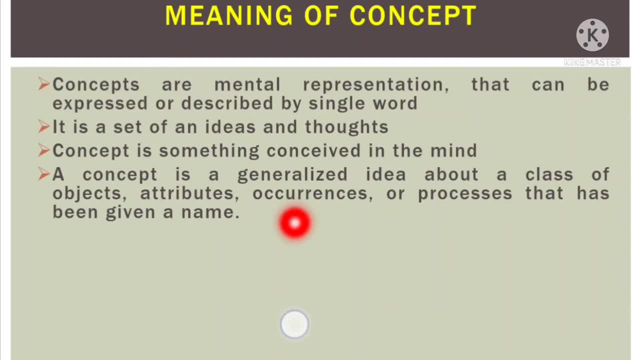 And when. what is happening Actually? what is happening in that thing, in that concept, Or what is being taught in it? What is occurring And process that has been given a name, Which is your process, What is the process of that concept? 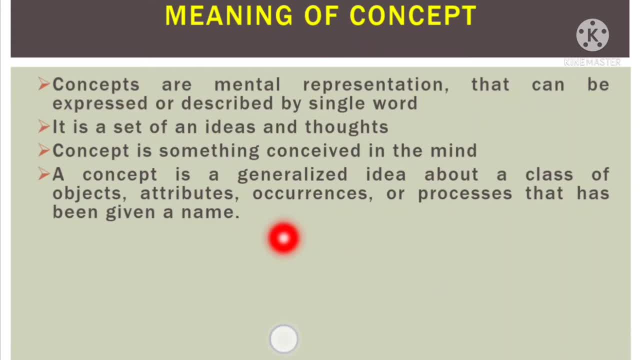 By combining all these things, we give a name to a concept in a journalised form That is called your concept. In other words, concept is expressed as a symbol or in words. It is simple that when we take any knowledge, we give it a name. 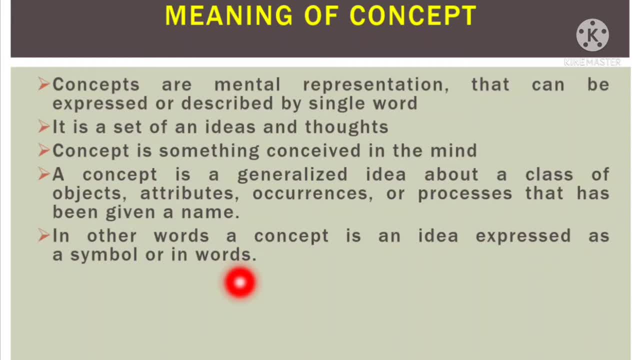 And that name is your concept: Force, Patience. What are all these things? These are words. If we explain them, then, what is it? The content of that particular concept is knowledge Right. A concept is generally accepted and understood. collection of meaning, characteristics associated with certain event, object, condition, people or behaviour. 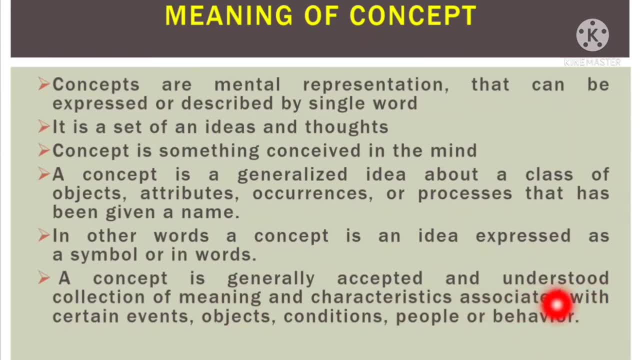 Every concept has its own characteristics. Every concept has its own characteristics, Every concept has its own meaning. So we have to accept it, We have to understand it And we have to apply it to the students So that we can bring change in the behaviour of the students. 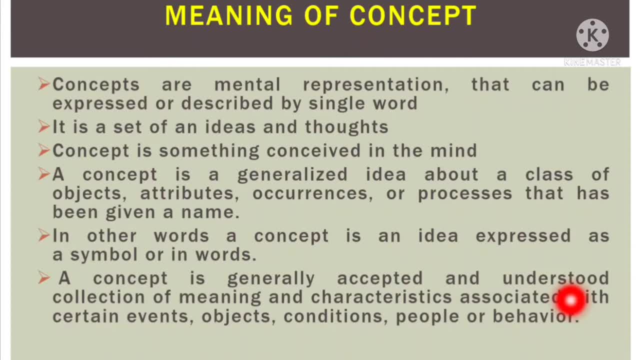 Whenever you learn a concept, whatever learning you do, you can see its reflection in your behaviour. Various sources of concepts. Your concept has many sources. Your source can be your teacher. Internet can be your source, Books can be your source. So the concepts that we form. we can learn the concept in different ways. 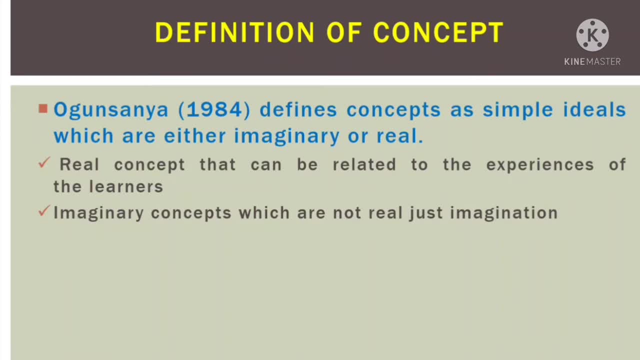 Ogunsanya defines concepts as a simple ideal, which are either imaginary or real. Now, here, in both imaginary and real forms, you can form the concept, You can frame it. What is a real concept? That can be related to the experience of the learners. 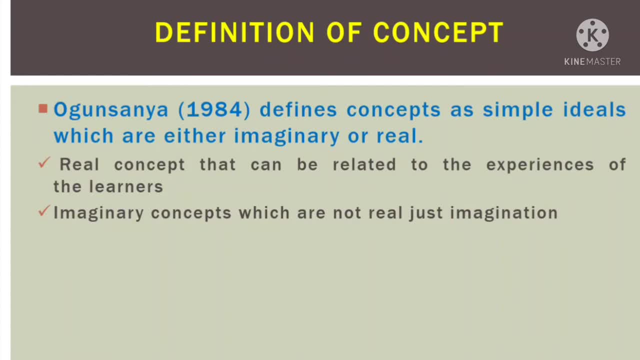 Here the real concept. whatever you are learning the experience of, that you are learning directly or indirectly. Sometimes in life we learn a lot from other people's experiences. Sometimes we learn the work by doing something ourselves. So what is the real concept? 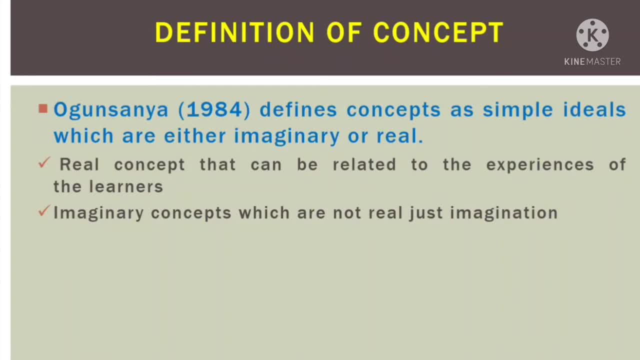 A real concept is learning from the experience of learning, the experience of learning its Энэєээ. The real concept is learning from one's experience. The imaginary concept is the one where some concepts are not real, just an imagination. 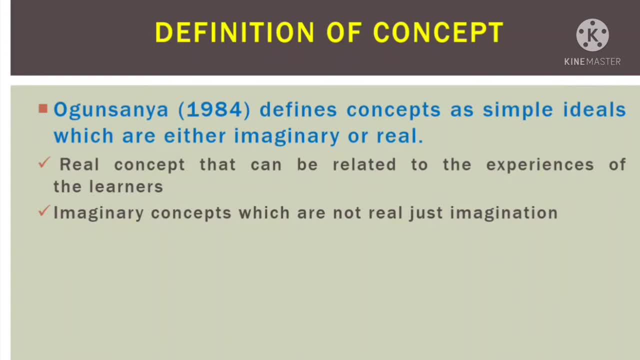 You can never have the same concept in our life. You can never have the same concept in your class. You have your own imagination and you think that we are forming the concept. Now is it going right or wrong? That is a different thing. 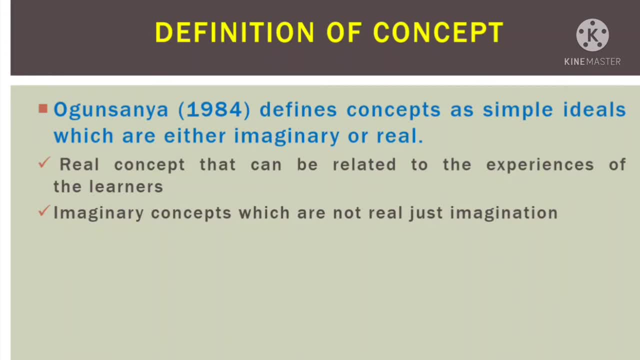 But with the help of imagination we can form a lot of concepts in life That we will do this in life. so that is your totally imaginary thinking, edgy boy. concept group thing into classes on the basis of their shared characteristics and they help us to distinguish one class from the another. so the most important thing about the concept is: 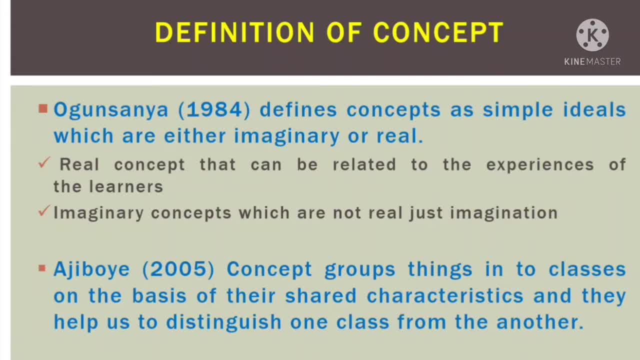 that we distinguish them according to their specialties. a concept is different from another concept. like we keep it simple here, talk about how your earth is different from your venus, so here the characteristics of the earth will be different from the characteristics of the venus concept. so we can differentiate them. 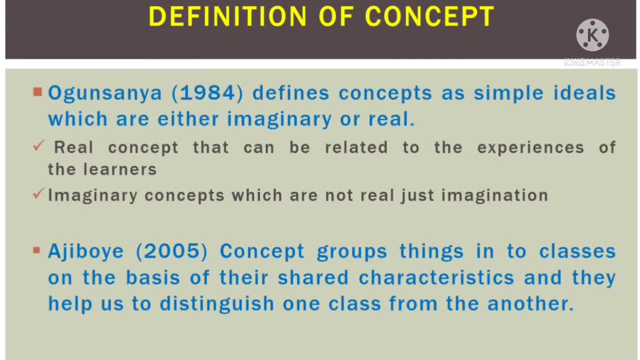 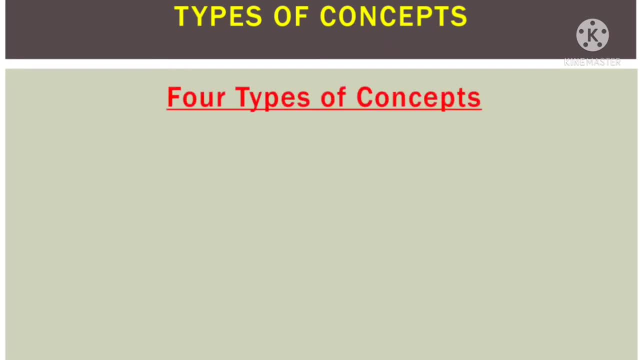 on the basis of their characteristics. next is types of concept. there are four types of concept. first is your concrete concept, which is called as thos avdharna in hindi. so the concrete concept is basically on the basis of common characteristics, that any idea which you want to generalize, but on the basis of its common characteristics. 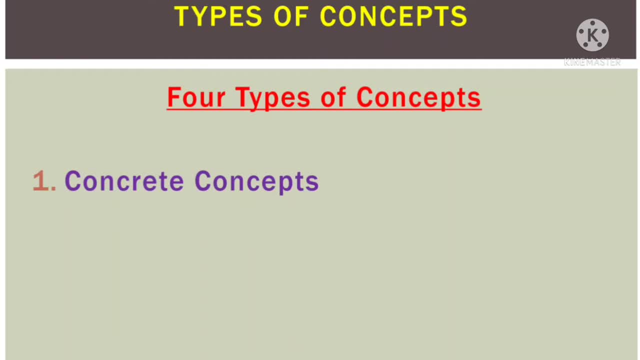 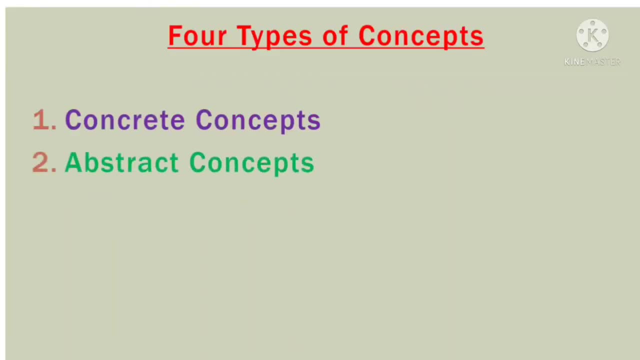 we are able to generalize that idea on the basis of what are the attributes, what are the specialties, what are the qualities? that concept will be formed on the basis of that abstract concept. these are imaginary concepts and they are basically something that we cannot feel or taste. for example, cooperation or unity. 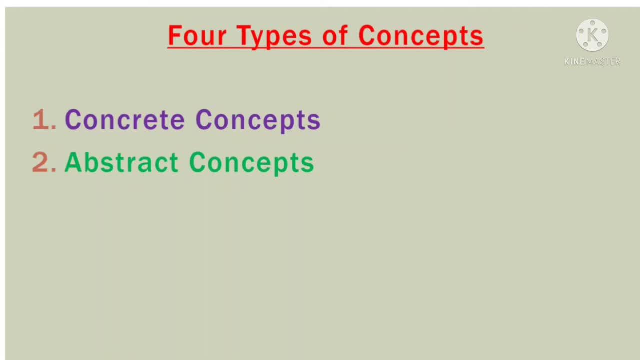 us okay is to radiation ac, but o can be cooperation and unity. ki feeling aapke andar hai, toh kai ki baad, jab koi aise activity hoti hai ya koi aisa attitude, aapka kisi perspective, kisi cheez ke liye aapko dikhana hota hai, 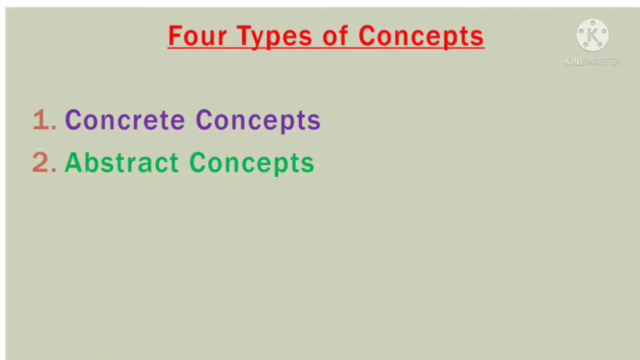 toh waha reflection aata hai aapke cooperation ka, aapke unity ka. toh ye cheez kya hai inbuilt hai aapke andar. isko aap perceive nahi karenge with the help of senses, but ye value aapke 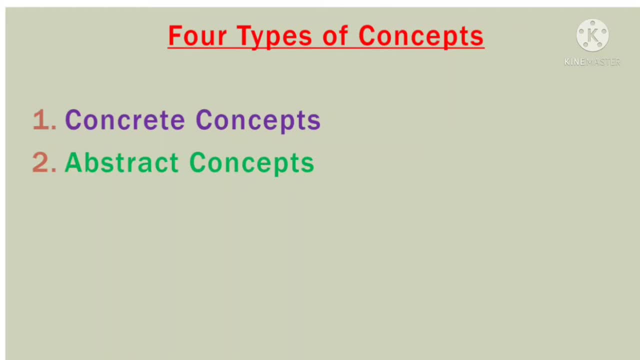 andar already inbuilt hai. concept of activities. next toyоронka concept of activities. gati vidyon ki avdharana, the concept making with the help of doing activities. yaa par kiya hai ki activities ka bohat bida role hai, ki jaab aap kisi kaam ko group mei koư individual activity kar. 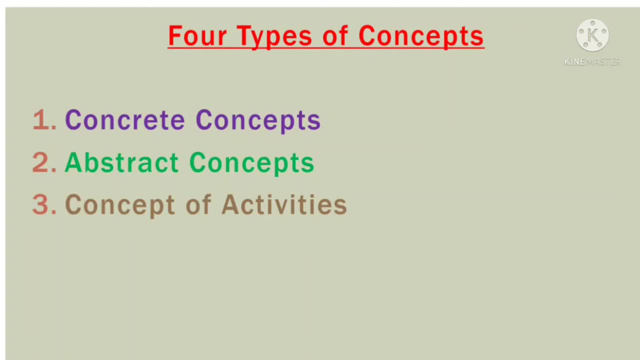 kar aap seek raha hai: studying, cooking, planning, playing yonki aap ki kaam가 ki basis aap liye toh aap, aap ki yonki aap lab smoking, drinking smoking and smoking in activities ke basis pe yon ekte orean ka shastra kar ke jaab ki aur external activities be wash pardoon. 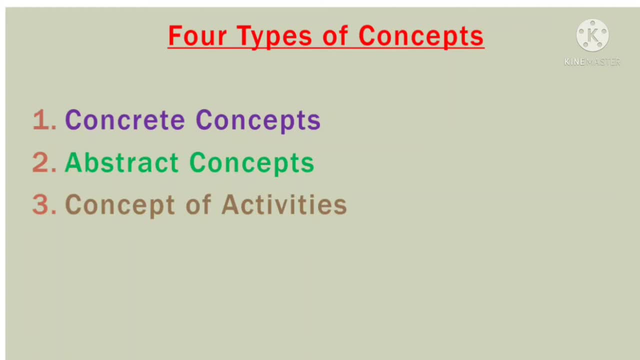 ki man mein ke wedding. kao will be doing so. ye sa funny. aap Из defini. logo is after an example. you don't know. we call it business, practical requirement. they used to call it personal, same primary. Your behavior is changing. It is simple. 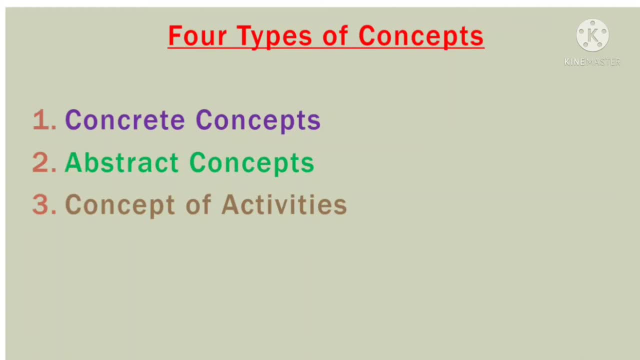 Because cooking is an activity, a series of related behavior organized into a sequence for the purpose of preparing the food. So here, when you are being taught about cooking, then a sequence has been prepared. Step by step you will learn cooking. you will know how food is made. 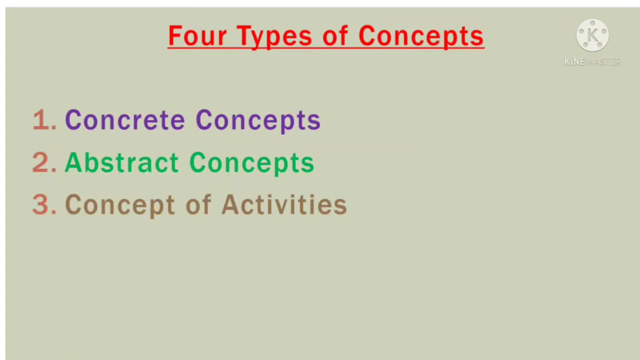 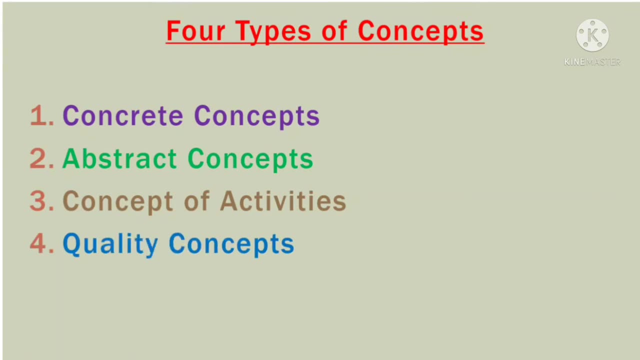 So here your behavior is being changed With the help of concept formation in a sequential form. Next is quality concept: gunavatta sampratya. We also have concept of quality- good, bad, better, poor- And there are many qualities which are inbuilt in us. 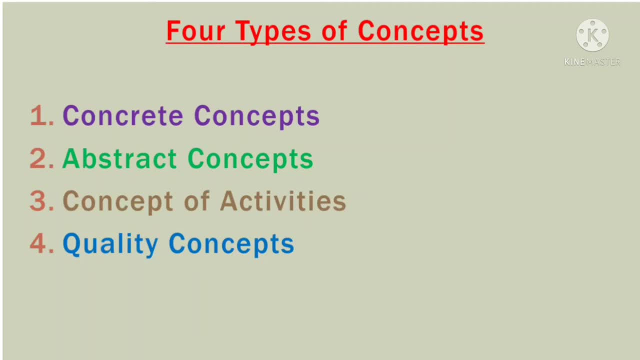 So here you can frame the concept on the basis of quality, As we talked earlier that you can frame the concept on the basis of characteristics. Similarly, you can frame the concept on the basis of quality. You can classify the concept. You can classify the concept. 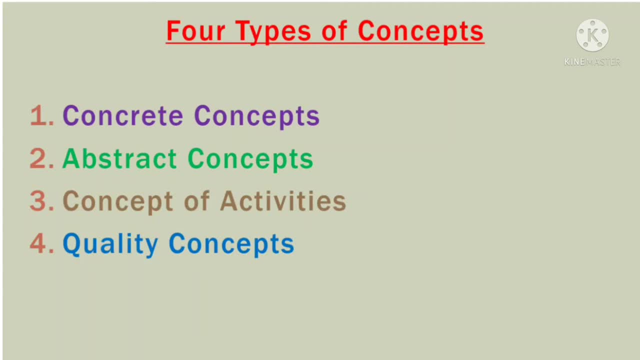 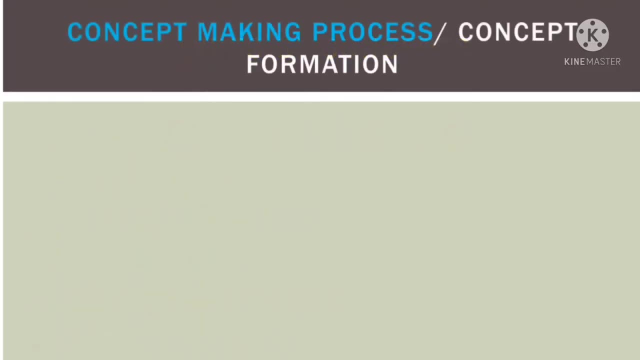 You can frame the concept on the basis of good and bad. You can frame the concept on the basis of essential and inessential. Next is our concept making process, concept formation. In psychology, making is the process of how people construct, understand. 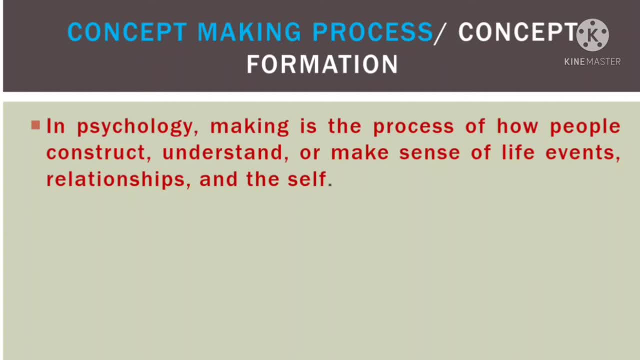 make sense of life events, relationship and the self. We have learned about concept making process till now. Now we will know how a teacher can form the concept in a classroom. By taking the child to an understanding level, they can change their behavior. 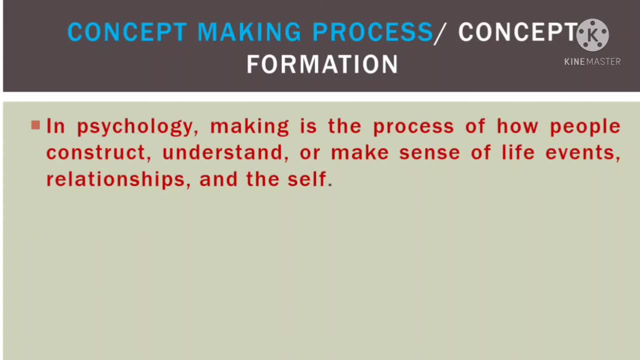 They can teach something new In psychology: making is the process of how people construct. First of all, it is important that the knowledge which you are learning, the process of the knowledge which you are learning, how it is constructed and made, You have previous knowledge. 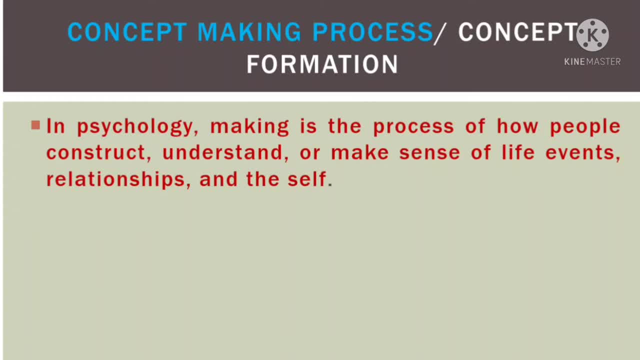 We are giving you new knowledge, So how you are constructing the previous and new knowledge. Understand the children and make sense of life events, relationship and the self. Whenever we form the concept, we try to connect you with real life events. 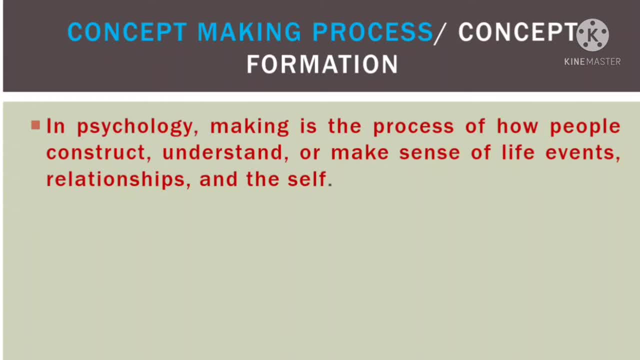 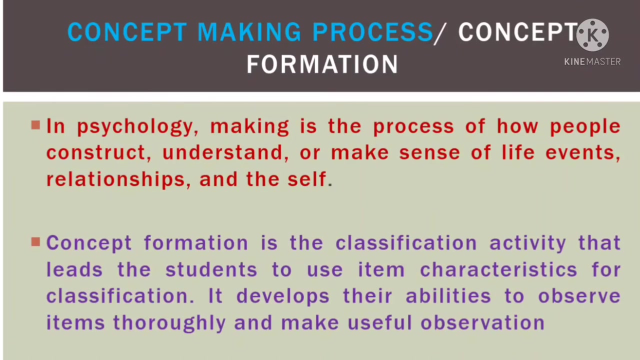 Use your senses, Because the senses are the gateway of knowledge. We use different senses to learn something. When we want to know what is the relationship between one concept and another concept, it is very important that there is a proper process. Concept formation is a classification activity that leads a student to use item characteristics for classification. 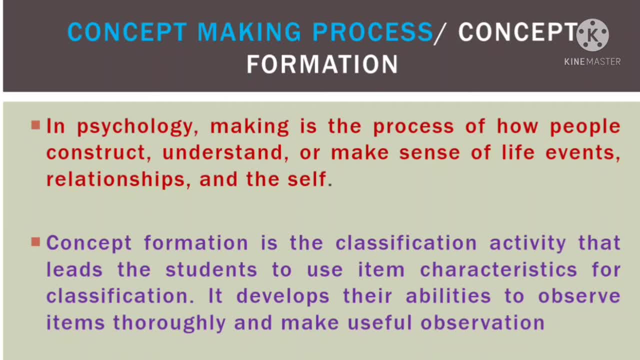 Classification is the process of making a concept. Classification is always done in the form of positive and negative, in the form of example or non-example, or in the form of essential and inessential. In our class, when we are teaching students, what will be the focus point? 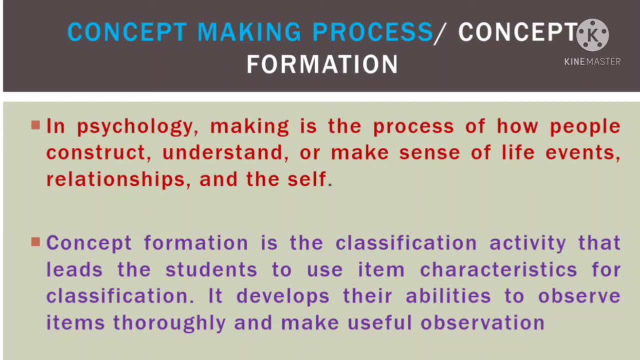 Along with the focus point. we have to give some non-examples in the classroom So that the concept of the children can be formed very well. So we have to keep the examples first, Non-examples at the time of explanation, We have to keep non-examples along with it. 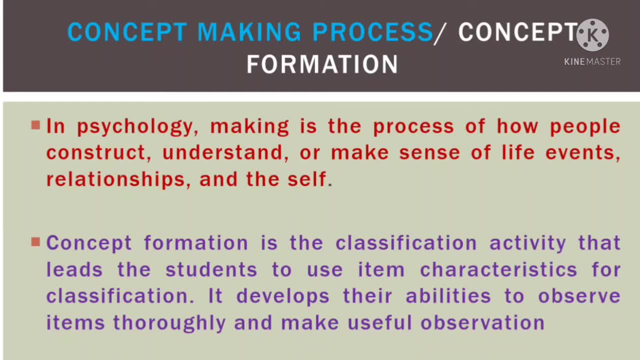 So that the children can differentiate between good and bad. It develops their abilities to observe items thoroughly and make useful observations. When you form a concept like this, first you give information. After giving information, we give knowledge to the children And, gradually, an understanding level. 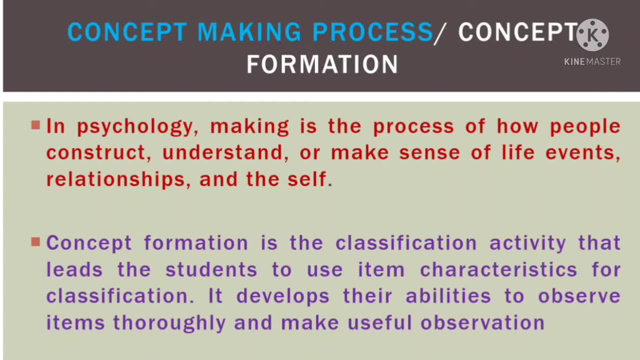 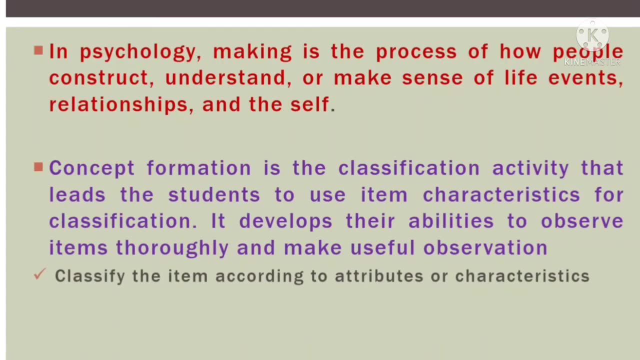 The deeper the children understand the concept. their understanding level develops, So an ability develops in them. They are able to observe things very deeply and thoroughly, Classify the item according to attributes and characteristics. The most important thing is whenever you form a concept. 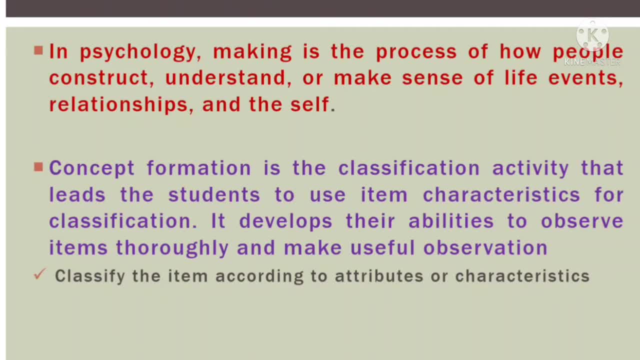 when you create a new concept, then you first separate the qualities and essentialities of the concept. On the basis of that, you first separate them, You classify them, What you want to keep first, what you want to keep later, What you want to focus on. 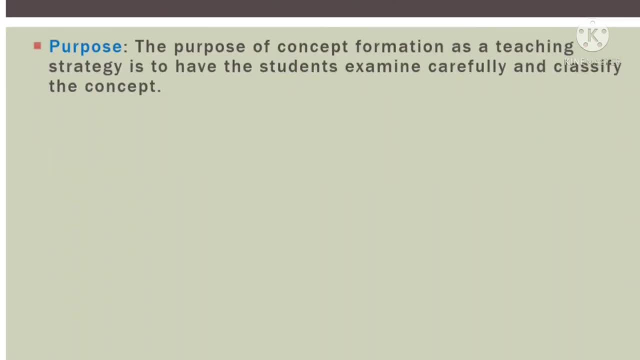 Next is purpose. What is the purpose of your concept formation? What are the objectives on which it is necessary to do it? The purpose of concept formation as a teaching strategy is to have the student examine carefully and classify the concept. When a teacher forms a concept in the classroom, 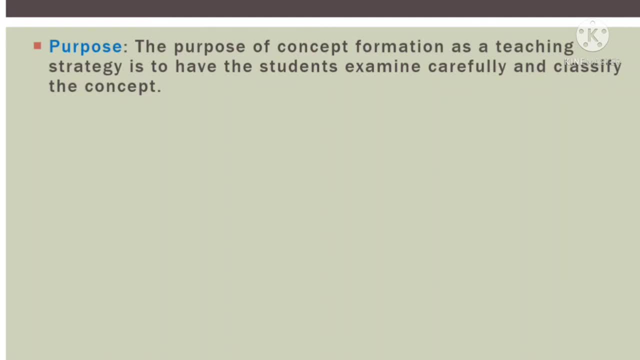 then it is necessary that the student understands it, That how they have to classify and divide their concept. It helps us to disregard what is inessential by creating idealized structure that focuses on what is essential. So when a teacher is forming a concept in the classroom, 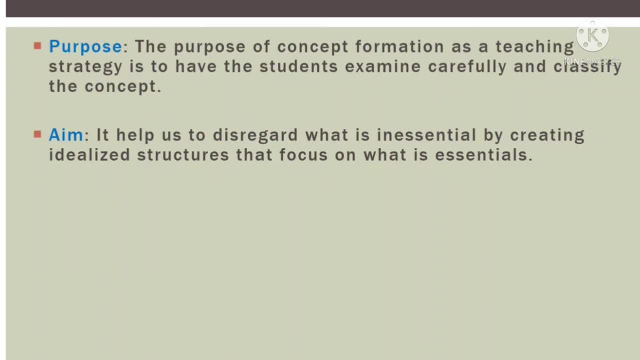 then the focus will be on focusing on essential things, And by using non-essential non-examples they also form the concept of the child. What are the advantages? Encourage certain of the common essential learning, like critical and creative thinking, communication and independent learning. 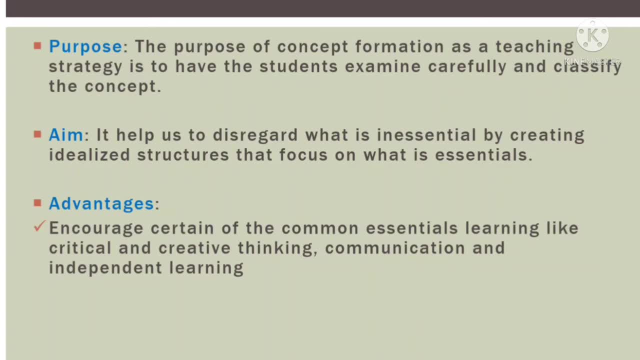 The benefit of concept formation is that here you can focus on which thing is more important, which is more important to learn And, critically, when you are able to know, you are able to judge that this is required and this is not required. 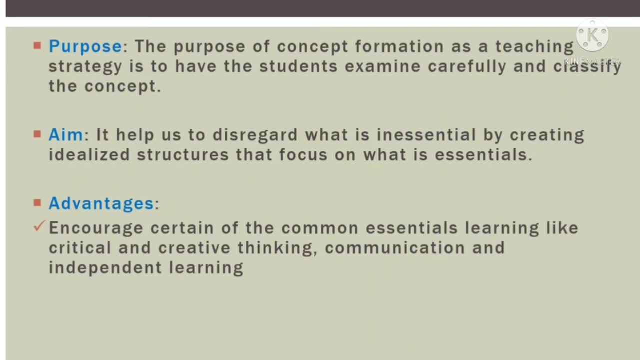 So here your judgmental skill, or you can say your creative and critical thinking, develops. You are able to share your ideas and thoughts, you are able to communicate and you are able to learn things independently. Here you have learned to judge what is essential and what is inessential in this concept. 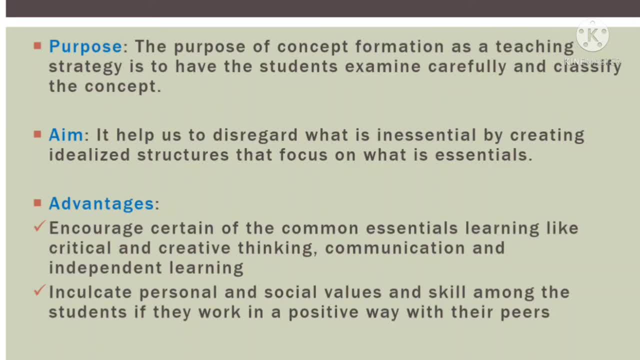 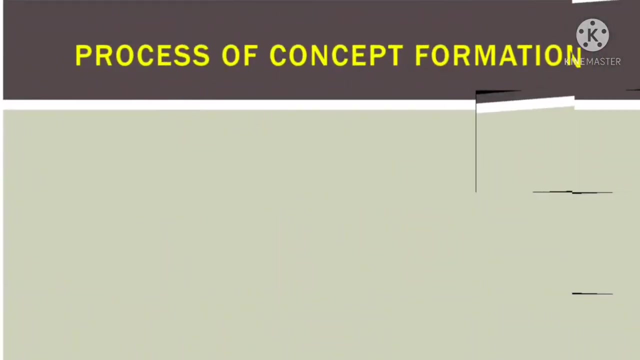 Inculcate personal and social values and skill among the student if they work in a positive way with their peers. Here both personal and social values develop And we learn a lot of things together with our peer group in a positive way. Process of concept formation. 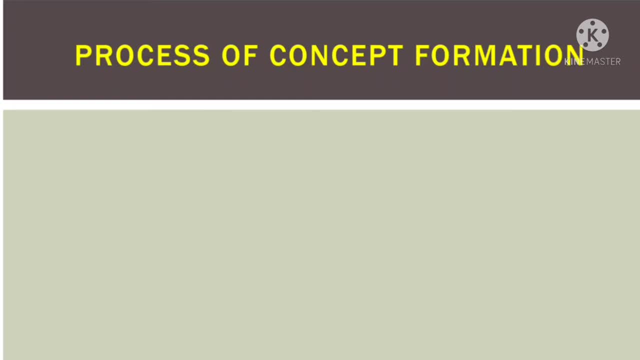 It is very important that when you are forming a concept in your classroom, you will not disclose the topic yet Today you have planned that you want to teach something new to the students, So here we will not announce the topic As soon as we announce the topic. 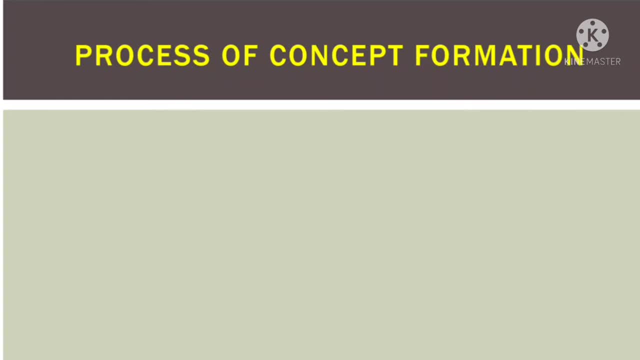 the students understand what we are going to talk about today. So right now we will make a ground. we will make groups of students. After making groups, gradually, we will take the students to that place On the basis of different explanations, with examples. 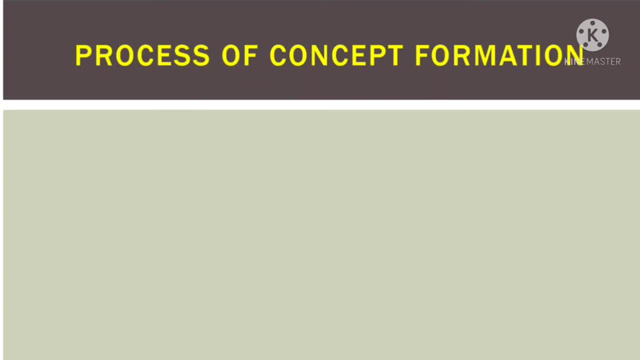 we will keep explaining our concept And after that we will ask the students: in the end, according to you, what is this topic today? So this way we will actually know whether the correct concept of the students has been formed or not. 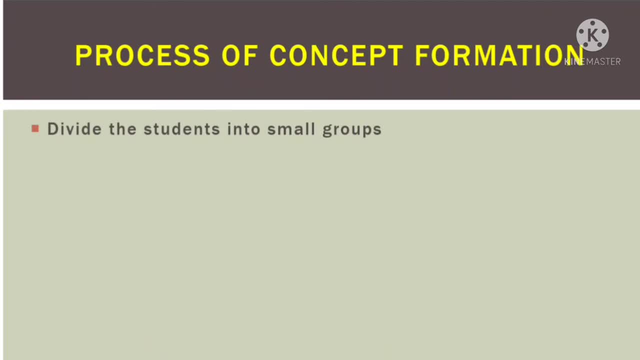 To form the concept, you will make small groups. Suppose you have 40 students in your class, then you can make a group of 10-10 students. You can make a group of 5-5 students. Provide the students with number of items to classify. 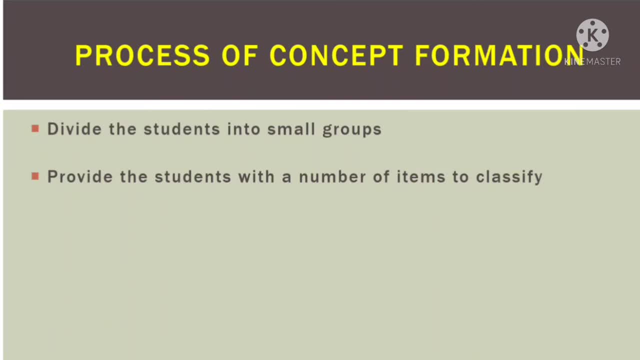 Now suppose you are teaching any topic to the students. As I told you, when we teach any topic, then its essential and inessential means in example and non-example we divide that topic. So what will the teacher do here? 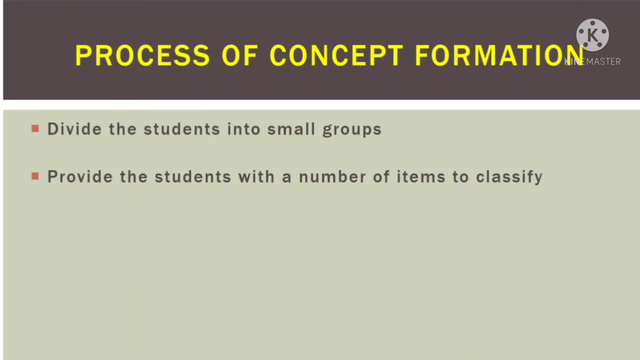 She will classify the examples and non-examples. Ask the students to organize the items into groups according to the characteristics of their choice. Suppose I have given you 7-8 items. Now I will show you an example how you can classify them. 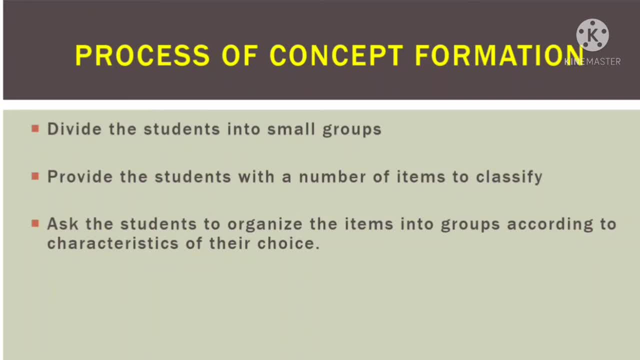 So here you will organize your items. You will give a lot of items to the students. Now what will the students do here? They will classify them according to their characteristics. When classification is complete, have each group explain their grouping rationale to the class. 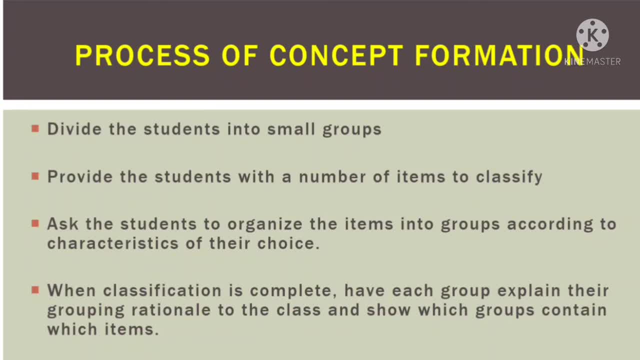 and show which group contains which item. So what will happen here? When you have given a lot of items to the students, you have classified them with the help of discussion that we have to keep them in example and non-example. So when the students classify, 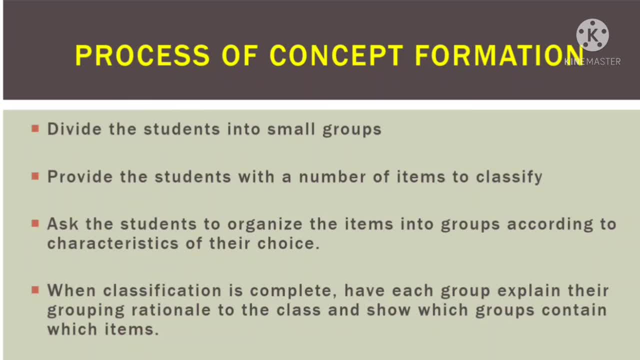 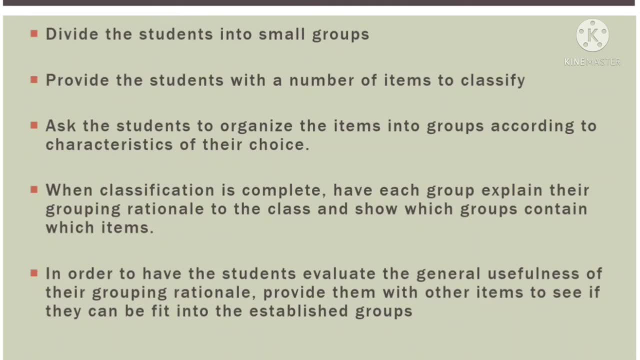 after that you can ask them on what basis did they do the classification and which one is kept in example and which one is kept in non-example. Now the students have classified, then it remains that the students will evaluate that, whatever they have learnt. 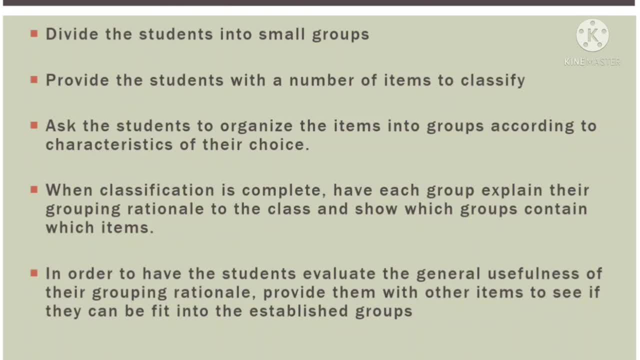 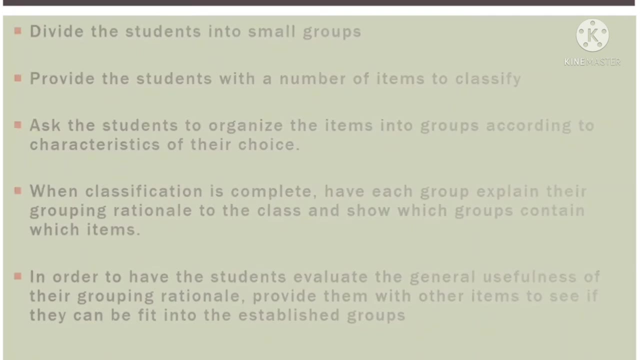 what was the fact behind it, what was the rationale, what was the reasoning? And if you give them more items, if their concept is formed, then definitely, if you give them more items, then they will be able to classify easily on the basis of their essentiality and their non-essentiality. 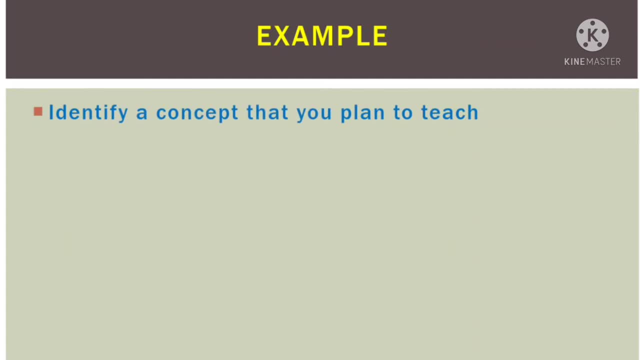 For example- I will give you a small example here- Identify a concept that you can plan to teach. First you identify the concept that what you want to teach in the classroom today. Then you give an example to the students, As I have written here. 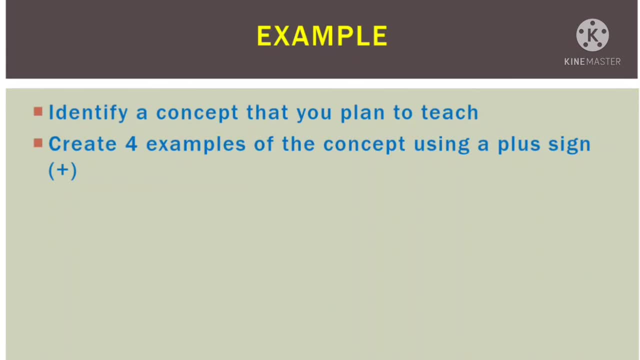 create four examples of concept. So four, five, six. there can be any number of examples. So the examples that will be here, the students will donate them with the plus sign. like obeying laws, paying taxes, casting votes. 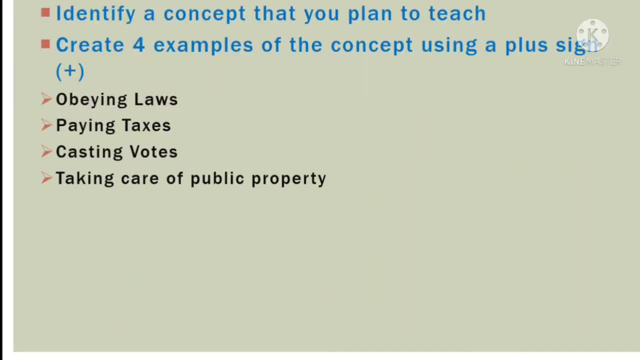 taking care of public property. So what is this? These are your positive, essential things that you have to teach the students in the classroom. Now there are three non-examples. How will you denote these non-examples With the negative sign? 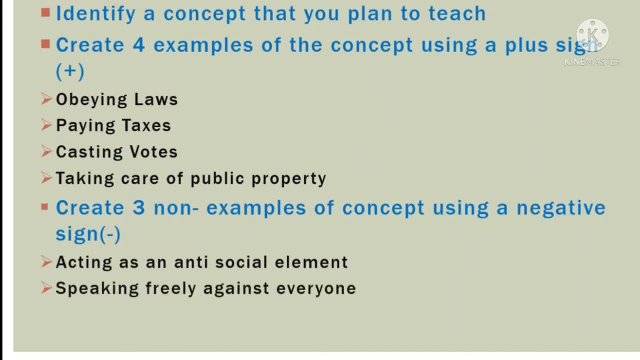 like acting as an anti-social element speaking freely against everyone polluting our surrounding. So what is this? When you explain four essential examples in the classroom, you will also bring non-examples so that the students understand what things they have to follow as a citizen. 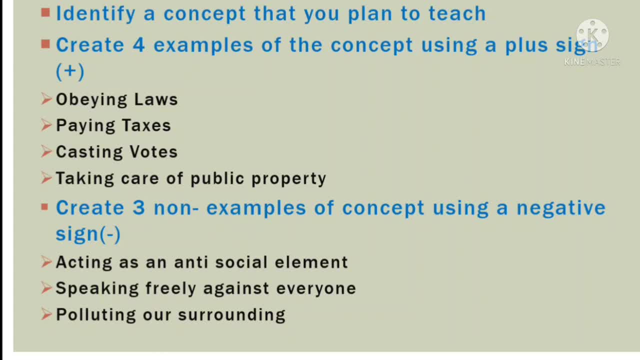 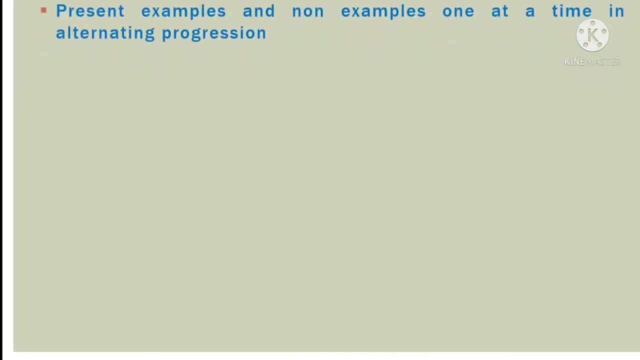 and what things they should not follow. I hope you have guessed what our topic is so far. Present example and non-example, one at a time in alternating progression, As I told you have the student guess what the concept is as each example or non-example presented. 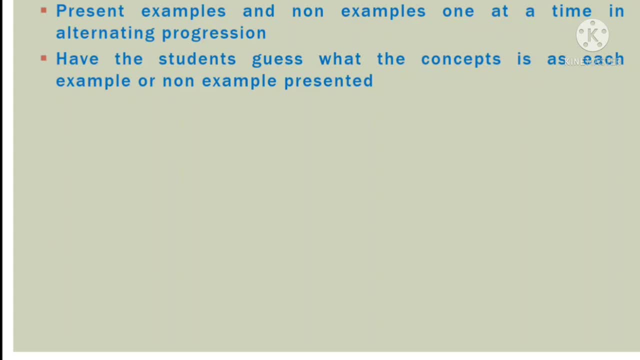 So now you will ask the students to guess that you tell us what is our topic today. according to you, You do not have to reveal your topic until you present it properly, And here you will be more focused on what will be your focus. 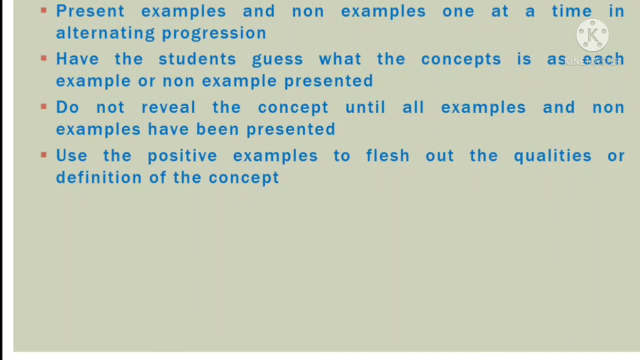 you will be more focused on positive examples, you will be more focused on its qualities. Then, when you present this way in the class, these students will do the full activity. After that, you will disclose what your topic is. So our topic was academic responsibility. 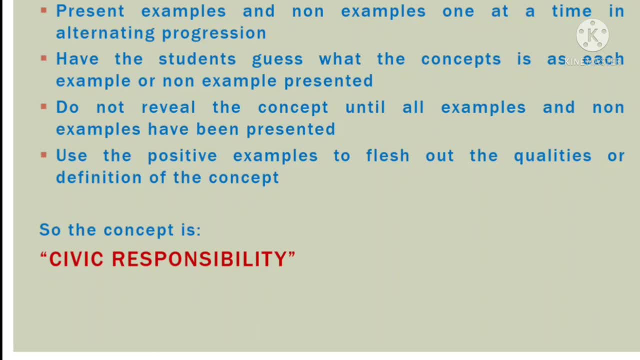 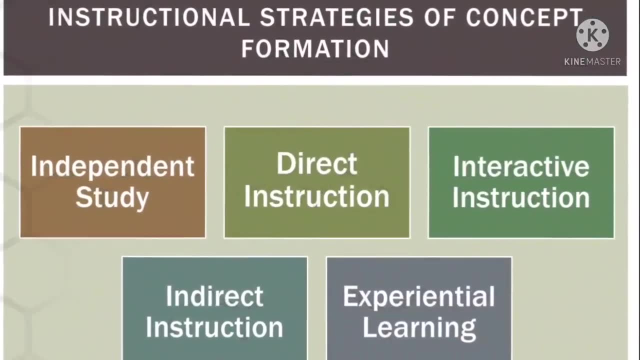 So this is very interesting for the students. It is real learning. They themselves can know what they have learned in the classroom today. Next is our instruction. Next is our instructional strategies of the concept formation. I will continue this topic in my next video. 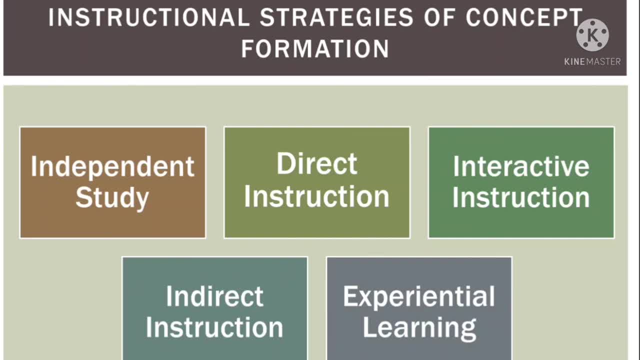 We will learn what are the strategies and what are the ways by which you can form new concepts in your classroom. So these are five strategies which we can use in our classroom. If you are interested, if you want to know more about concept formation. 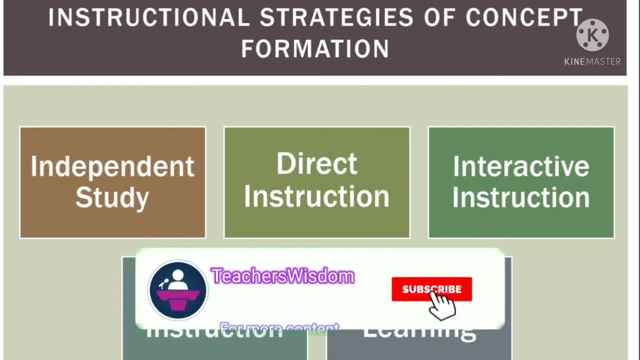 then you can subscribe to my channel. Whenever I upload a video of instructional strategies, you will get a notification. You will get to know first. You can also click on the bell icon so that you will get a notification that, yes, my new video is uploaded. 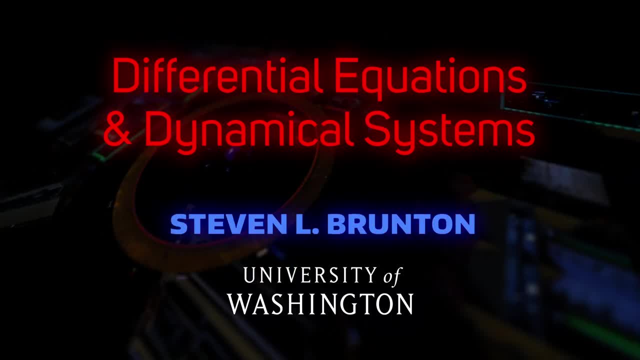 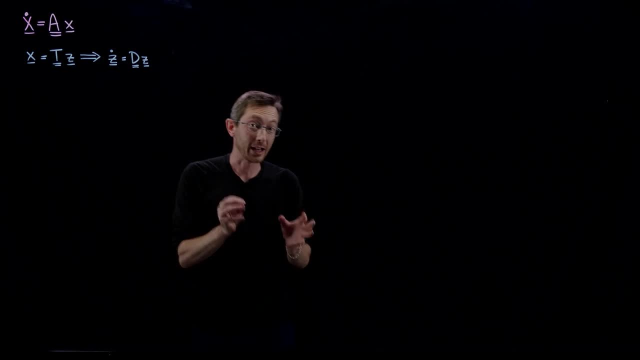 All right, welcome back. So this is the third lecture on the series of eigenvalues, eigenvectors and how to solve systems of differential equations. This is one of my absolute favorites because this is where it all comes together, So I'm staying late just for this lecture. 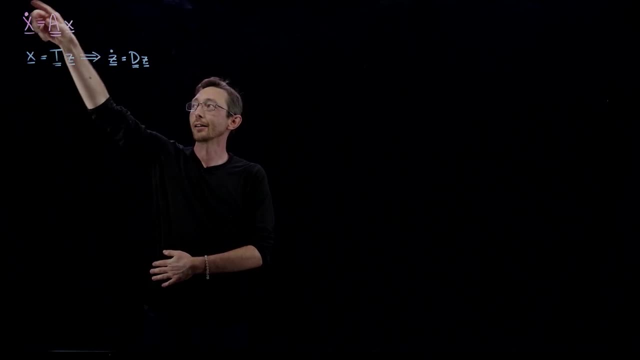 In the last few we have talked about why we have, you know, these ordinary, these systems of ordinary differential equations: x, dot equals ax, x is a vector, a is a matrix and these dynamics are coupled. But it's a lot easier to solve this system of equations if a 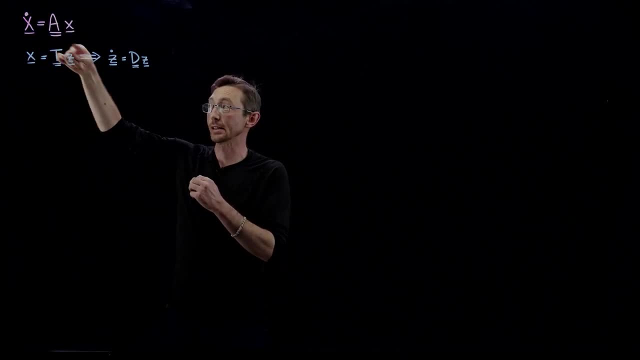 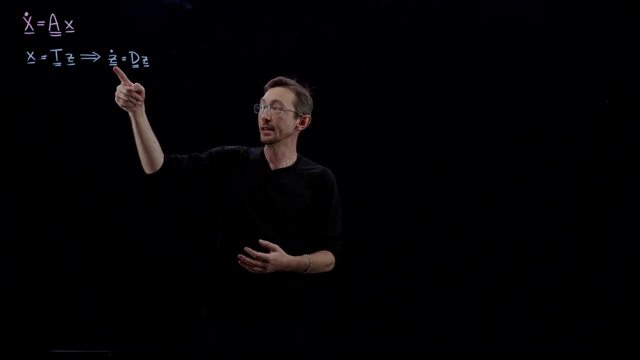 was a diagonal matrix. So we try to find a coordinate transformation, some matrix T, some invertible matrix T into some new coordinate system z, so that z, dot equals a diagonal matrix z, Because this is way, way easier to solve this system where d is diagonal and the